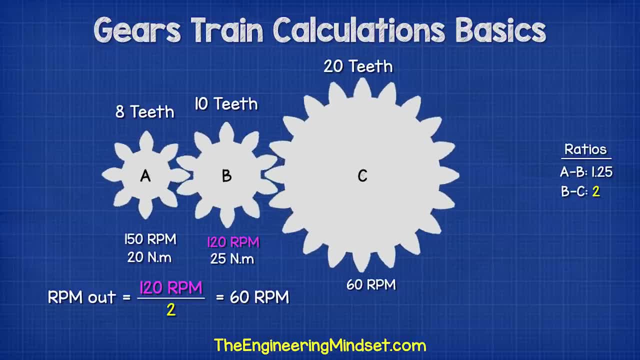 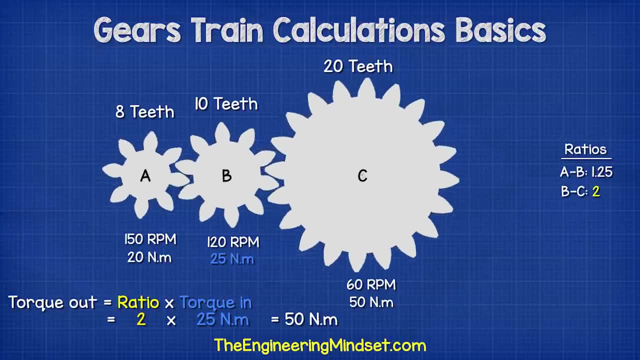 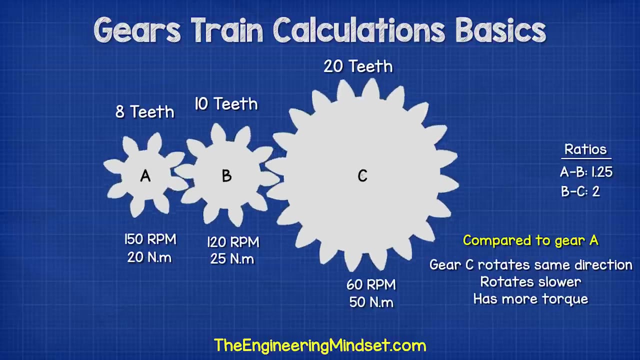 The RPM output is 120 RPM from gear B divided by 2, which gives us 60 RPM. The torque is going to be 2 multiplied by 25 Newton meters from gear B. This will give us 50 Newton meters. So this gear will rotate the same direction as gear A, but it will rotate slower. 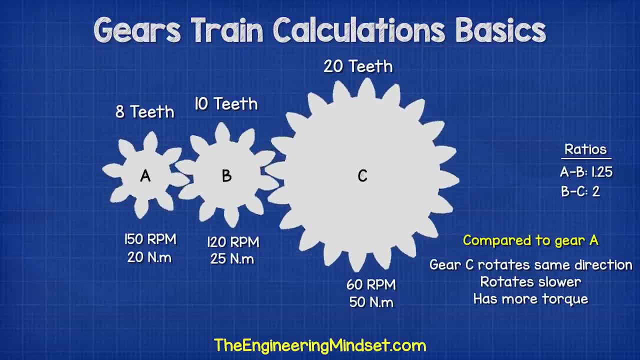 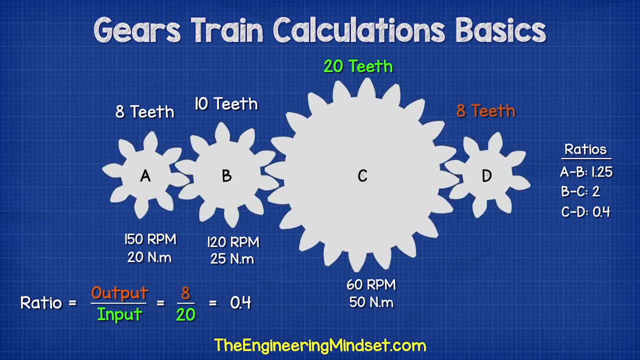 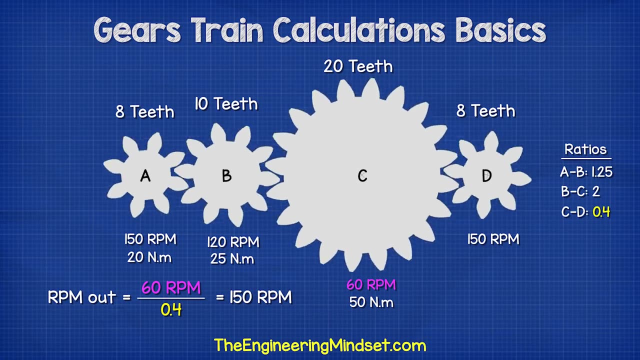 because it is larger, although it will have more torque. If we were to add gear D with 8 teeth, then the ratio is 8 divided by 20, which gives us 0.45.. The RPM is 60 RPM from gear C divided by the ratio of 0.4, which gives us 150 RPM. 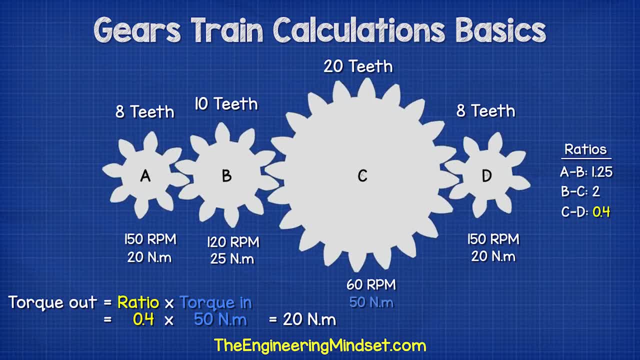 The torque is 0.4 multiplied by 50 Newton meters, which gives us 20 Newton meters. So this gear will rotate the opposite way to gear A, but it is the same size, so it will rotate at the same speed and the same. 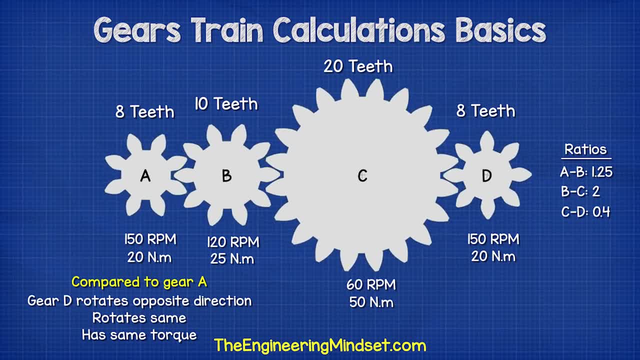 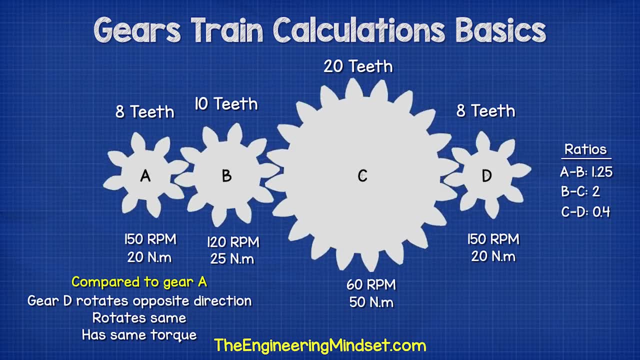 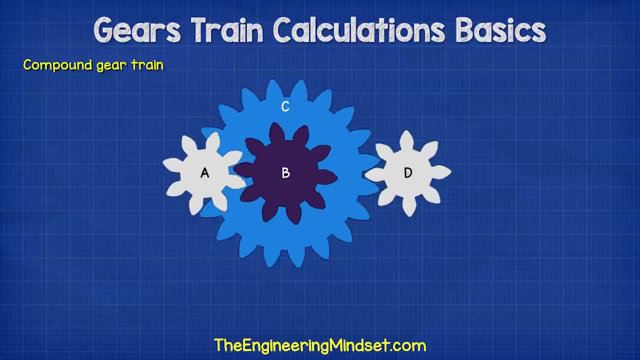 torque, although this doesn't take into account any losses which we would see in the real world. So this setup lets you visualize how gears manipulate speed, torque and direction. What if we had a compound gear train like this which has the same size gears? 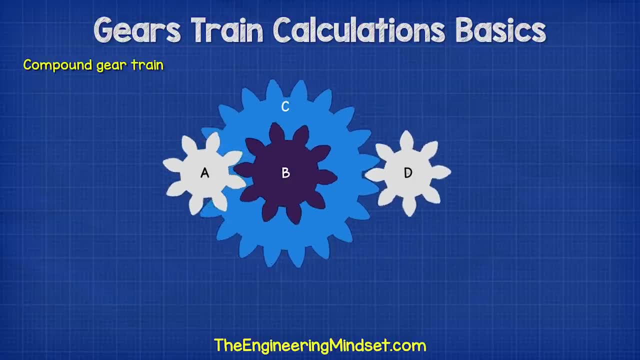 the same input torque and the same rotational speed. Again, links in the video description for the Excel sheet calculator for this. So with this setup we have four gears: A, B, C and D. but B and C are compound If gear A has 8 teeth and gear B has 10 teeth. 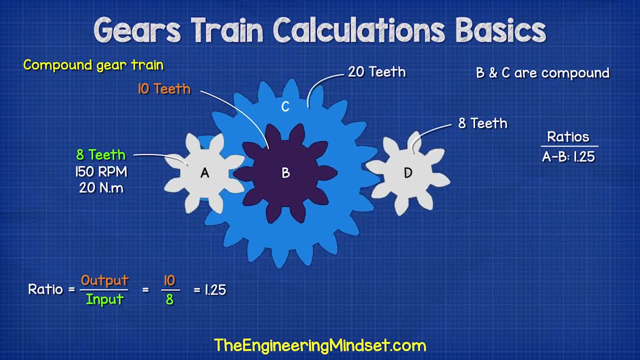 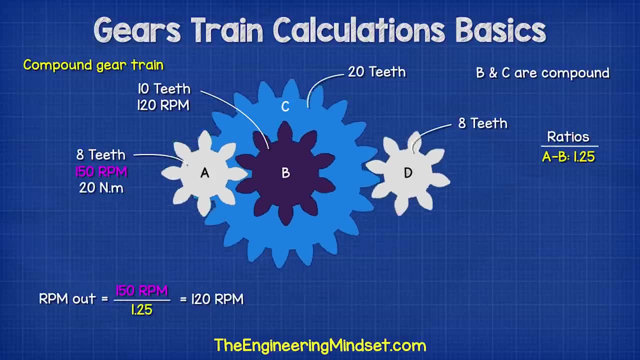 then the ratio is 10 divided by 8, which is 1.25.. Gear A rotates at 150 RPM, so gear B is 150 RPM divided by 1.25, which gives us 120 RPM. Gear A has a torque of 20 Newton meters, so gear B is 1.25. 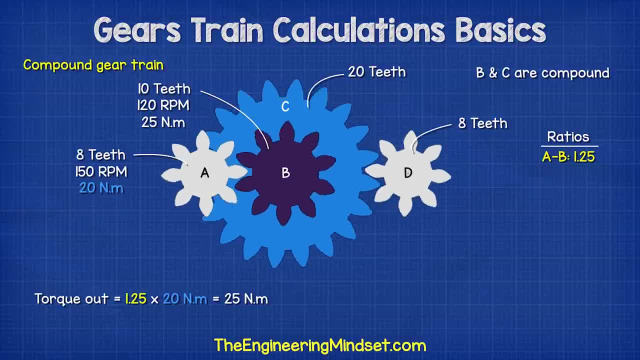 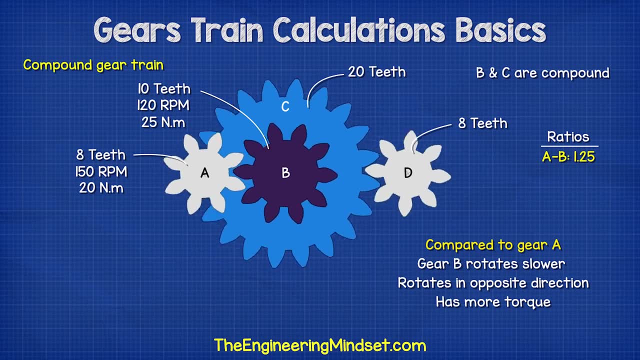 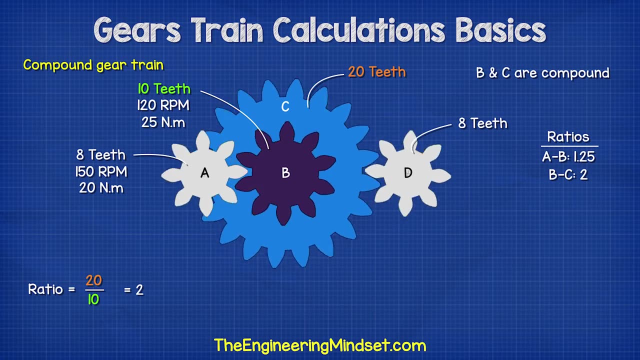 multiplied by 20 Newton meters, which is 25 Newton meters. So this gear rotates the opposite way to gear A. It will rotate slower because it is larger, but it has more torque. If gear C has 20 teeth, then the ratio is 20 divided by 10, which is 2..